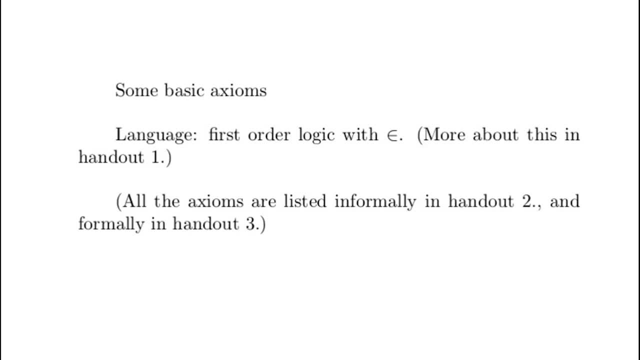 The axioms- all of the axioms, by the way, are listed in handouts two and three, informally in handout two and formally in handout three. So the handouts are extra text that you can refer to if you want to and they will be on the course materials section of the website. 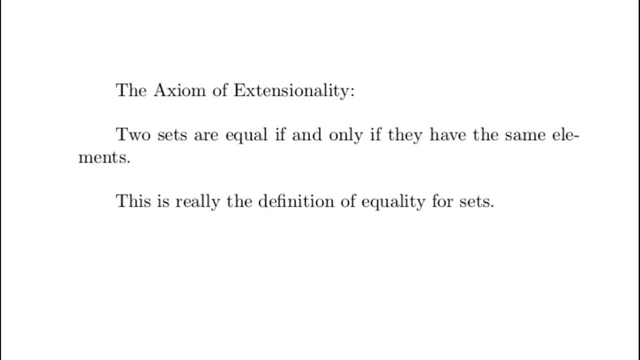 Okay, first, the axiom of extensionality. I should say that it isn't at all obvious that the axiom of extensionality should be regarded as true. Two sets are equal if, and only if, they have the same elements. In ordinary life this is weird. So in ordinary life we might say we would end up saying: 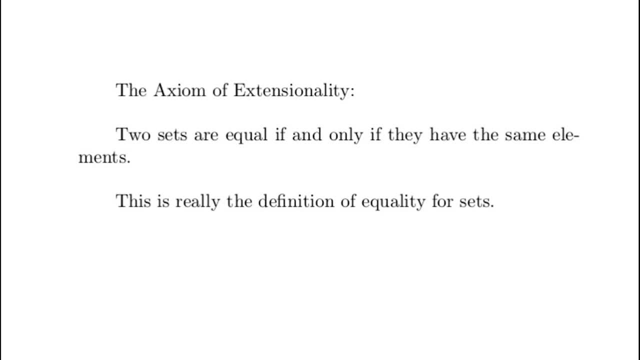 that the set of vampires is the same as the set of vampires. So the set of vampires is the same as the set of vampires. So the set of vampires is the same as the set of vampires. So the set of vampires is equal to the set of mermaids, because there aren't any of either. This seems weird If you're. 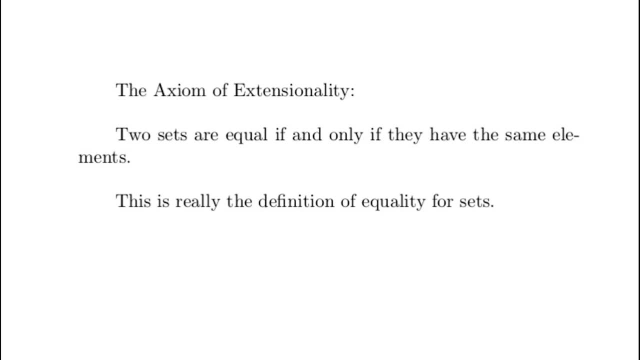 a philosopher, you may have heard of intentionality, and the reason we- perhaps a reason we- regard saying that the set of vampires is equal to the set of mermaids is that we can imagine a world in which that isn't true. So we can imagine a world in which the set of vampires is equal to. 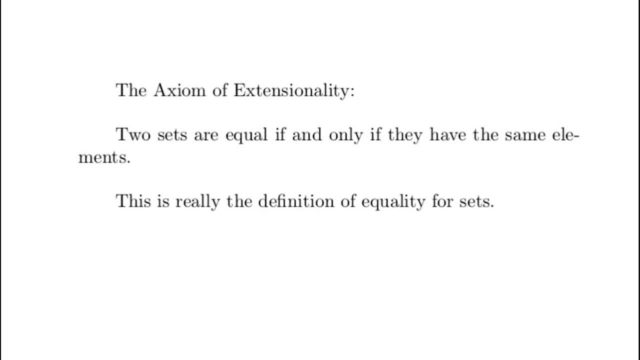 the set of mermaids is equal to the set of mermaids is better than the set of mermaids is equal to that. Okay, so what? the axiom of extensionality is really the definition of equality for sets and for pure sets it works, And so we're going to say that two sets are equal if, and only if. 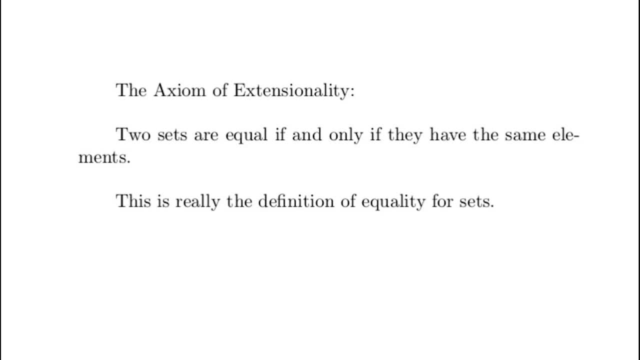 they have the same elements. Okay, the empty set axiom. We don't need this from the axioms of first order, false. So the axioms of first order, false are going to say that set of vampires is equal to logic and the other axioms we can actually deduce it. but whatever, we will say it because 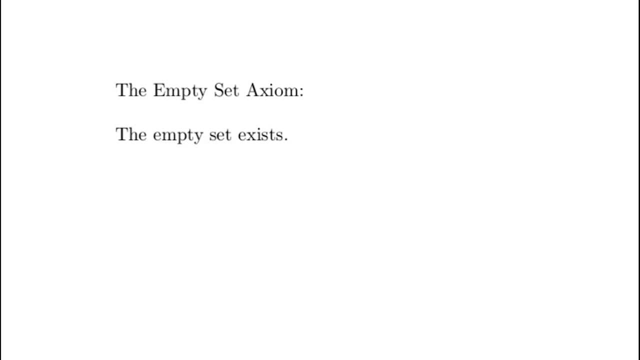 it flags it up as important. the empty set exists and therefore, in particular, there exists some sets, okay. next, the axiom of pairs. this is the first of a whole series of axioms that allow us to build more complicated sets out of simpler ones. okay. the axiom of unions sort of goes in the other. 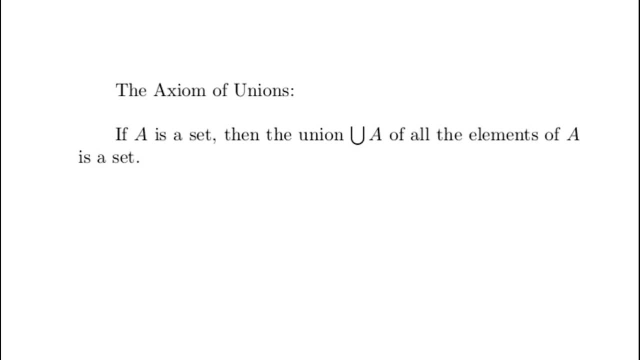 direction. if a is a set, then the union of all the elements of a is a set. so if you hand me a box full of a bunch of parcels, i can unwrap all the parcels and put the contents in a box. so, um, so, if so, the union of all the elements of a. there is a sense in which it's. 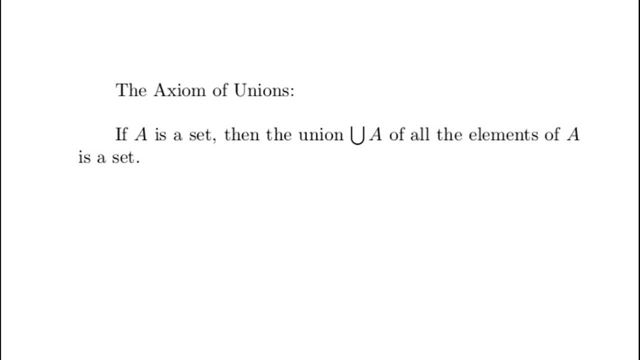 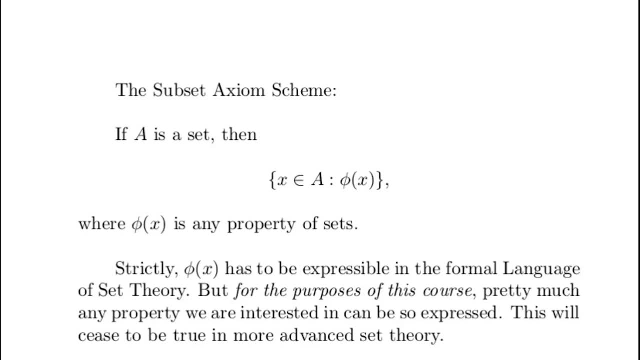 one level lower in complexity than a itself, the subset axiom scheme. so this isn't one axiom, it's infinite set of them. if capital, a, is a set, then set all elements of a satisfying a property, phi, that's a set as well. okay, um, okay, this, this, this set of axioms, um. 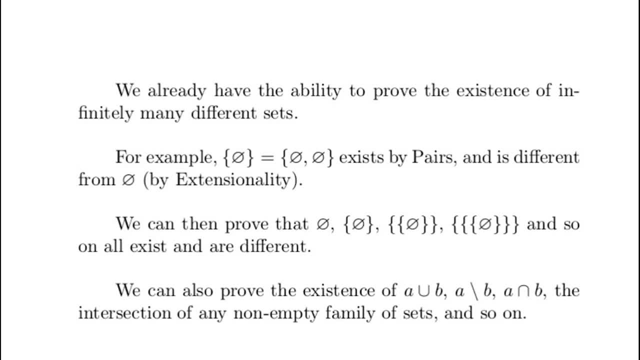 we already construct a load of different things, So I talk about some of those. in the lecture notes I'm just picking out a few examples for this video. The set whose only element is the empty set exists by the axiom of pairs. because when I stated the axiom of pairs, let's have another. 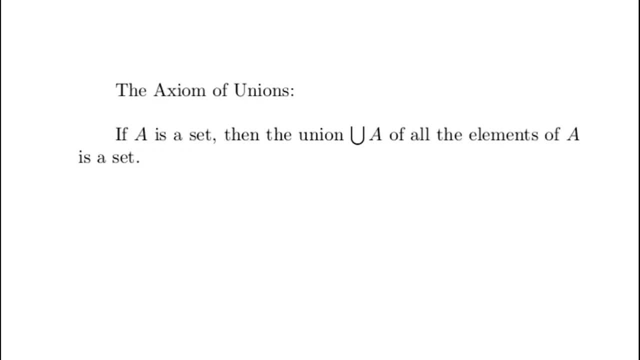 look at it, That's not it. this is When I stated the axiom of pairs. I didn't say that a and b should be different. they can be the same. So the set whose only element is the empty set is a set. 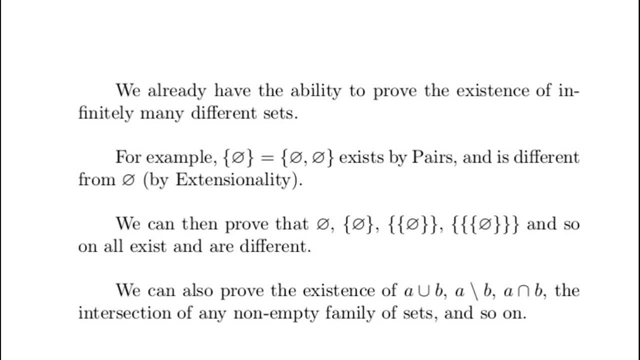 and is different from the empty set itself. Why? Because it has a single element and therefore isn't empty. Okay, so I can carry on putting pairs of curly brackets around and end up with a sequence of sets where it's possible to prove that they're all different. 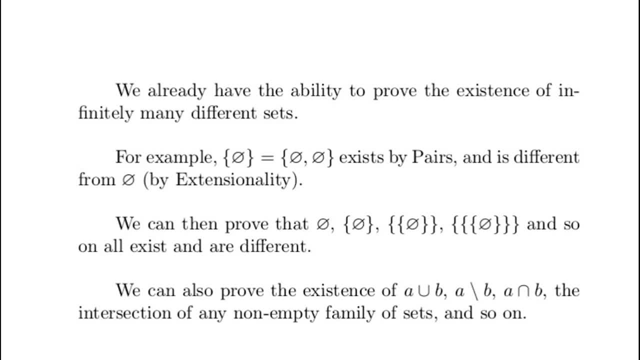 So we've got infinitely many different sets And we can also define union of two sets, the set difference. we can define intersection, The union of a and b is you apply the axiom of pairs to a and b to get the set whose elements? 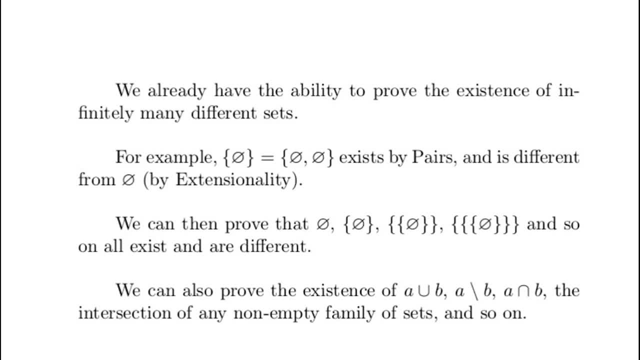 a and b. take the union of all the elements of that and we get a union b, And the other two sets can be defined as subsets of a union b. Okay, so we can do a lot of stuff with the axioms we've got already. There are things that we can't.